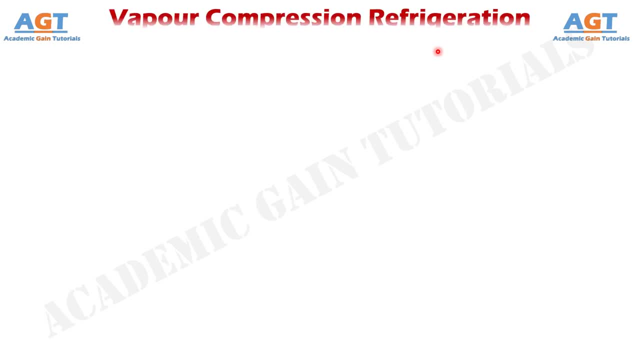 Welcome to Academic Game Tutorials. In this video, we will learn about the Vapor Compression Refrigeration System, along with its different parts and functions. So let's get into the topic. We know that refrigeration is the process of lowering the temperature by removing 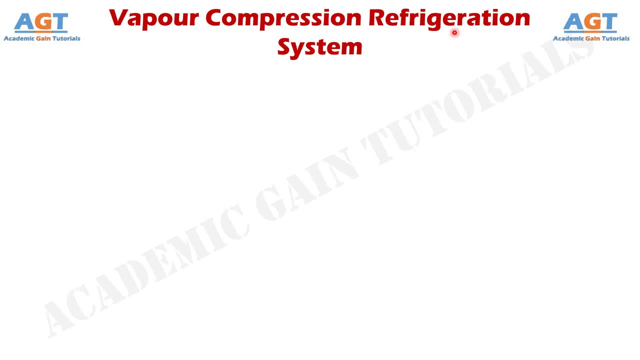 unwanted heat from a selected object, substance or unenclosed space and transferring this heat to another object, substance or space. Now, from the name Vapor Compression Refrigeration System we can understand that in this process we will compress a vapor refrigerant inside. 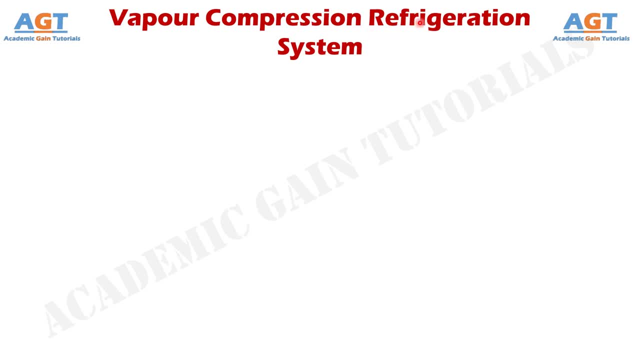 the system to obtain the refrigeration or cooling. If we are going to compress vapor in this system of refrigeration then obviously we will need a compressor for this job. So the process of compressing the vapor refrigerant inside the system using a compressor to obtain 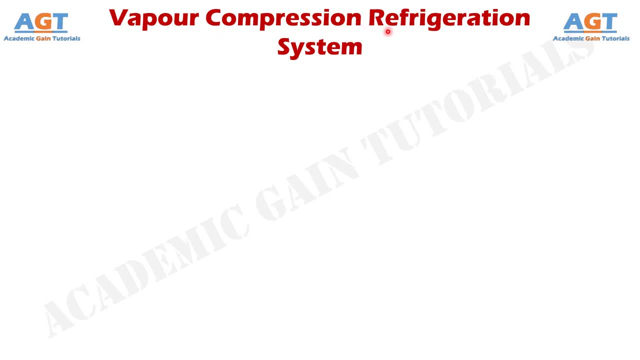 the refrigeration or cooling is called Vapor Compression Refrigeration System. Now let's look into the major parts and components and basic working procedure of the Vapor Compression Refrigeration System. So here we have a compressor, after that there is a condenser, then there is an expansion valve or throttle valve, or we can simply call 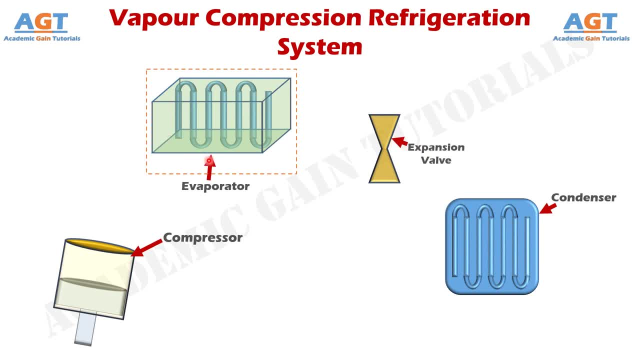 it a valve and finally there is an evaporator. So these four major components together construct the Vapor Compression Refrigeration System. All these components are connected to a vapor and are connected together using these connecting pipes. thus a closed loop system is formed. 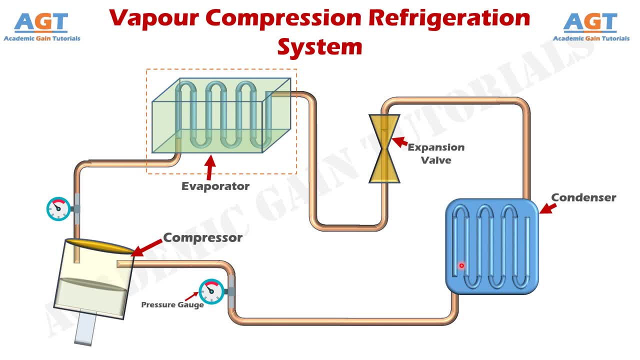 and the refrigerant for this Vapor Compression Refrigeration System will flow through all these components and pipes in the system. Now let's see how these components work Throughout the whole process. our main purpose will be to ensure that continuously cooling effect or refrigeration effect is obtained in this evaporator. We all know that this 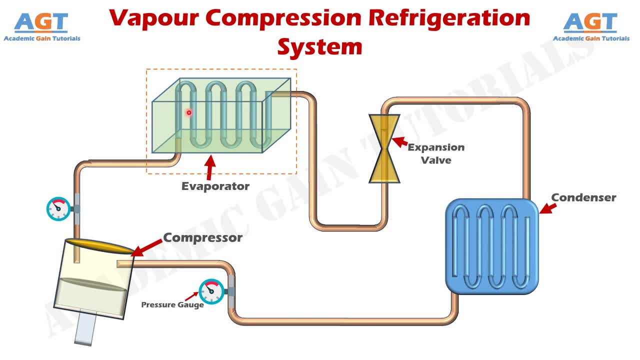 evaporator is the component where the refrigeration or cooling actually takes place. So we can see that this evaporator is placed on the region where we need cooling and then the evaporator absorbs all the heat of that region and passes those heat to the cold refrigerant. 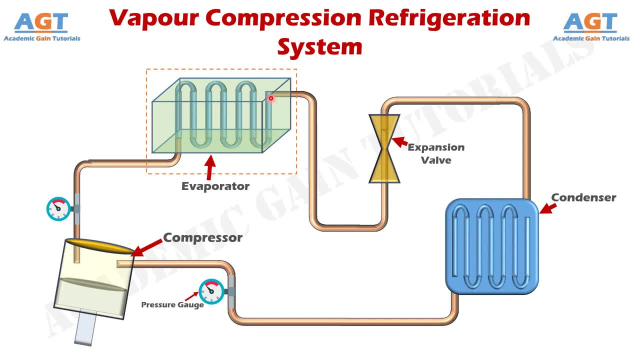 passing through the evaporator coils. thus the surrounding environment cools down. So let's see how this process works. First of all, this compressor starts working. The job of the compressor is to pressurize or compress the vapor refrigerant inside this compressor. 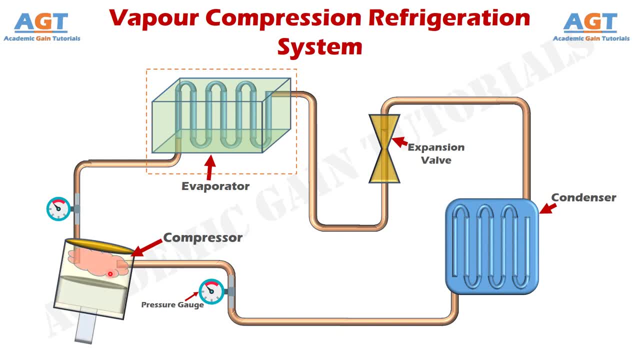 chamber. Here in Vapor Compression Refrigeration System we commonly use either ammonia or freon as a heat carrying medium throughout the whole procedure. Now we know that if pressure increases, it also increases the temperature. So when this vapor refrigerant is compressed inside, 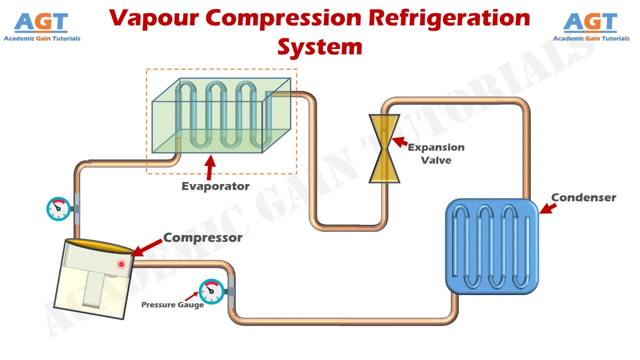 the compressor chamber by squeezing the vapor very tightly together. it will heat up. After that, this high pressure and high temperature vapor refrigerant will leave the compressor and will enter into the condenser. Here we have a condenser When high temperature, high pressure vapor refrigerant enters. this. 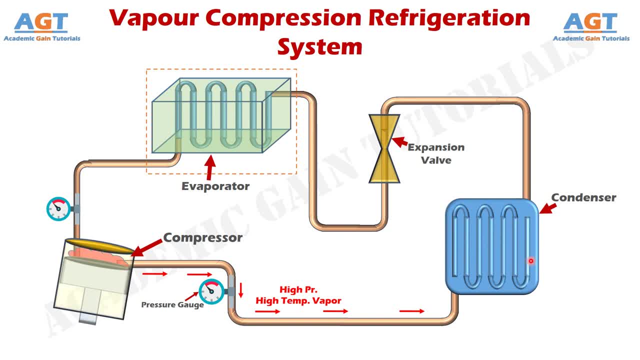 cold condenser, then the condenser absorbs the heat from the vapor refrigerant and completely converts it into liquid. This condenser can be water cooled, air cooled or cooled by any other substance from an external source which will liberate the latent heat of this. 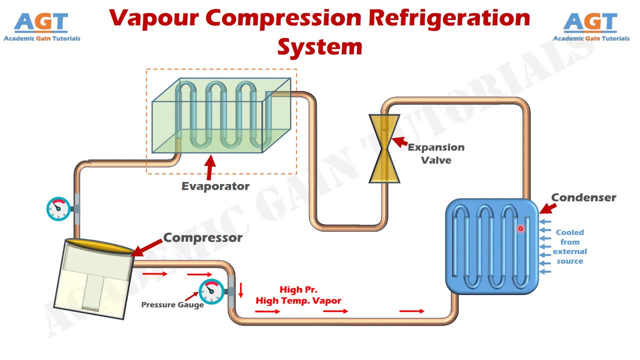 vapor coming into the condenser and thus condensing keeps happening. So in easier words, this is a cold condenser. Here we have a condenser. In this case, condenser changes the incoming high temperature, high pressure vapor refrigerant into liquid state by changing its phase. Here we had vapor coming. 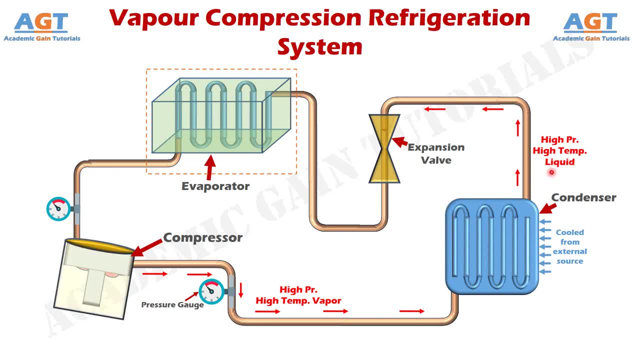 in and now we have liquid refrigerant going out. so the phase is changed. Now this high pressure, high temperature liquid refrigerant will leave the condenser and pass through this expansion valve or throttle valve, using this connected pipe. Now this high pressure. 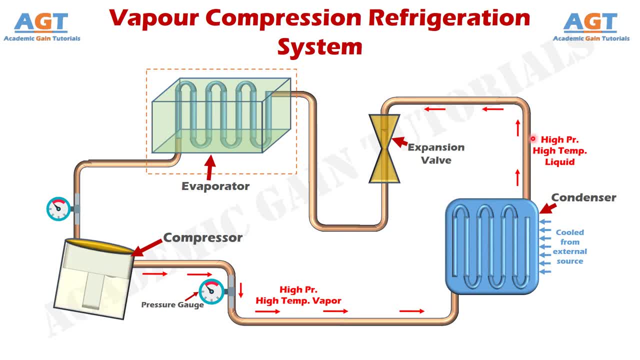 liquid refrigerant coming from the condenser will be expanded inside this expansion valve. Know that when expansion occurs the pressure between the molecules decreases considerably. thus the temperature falls. So this high pressure liquid refrigerant will be expanded into low pressure, low temperature liquid refrigerant In practical use at this point, 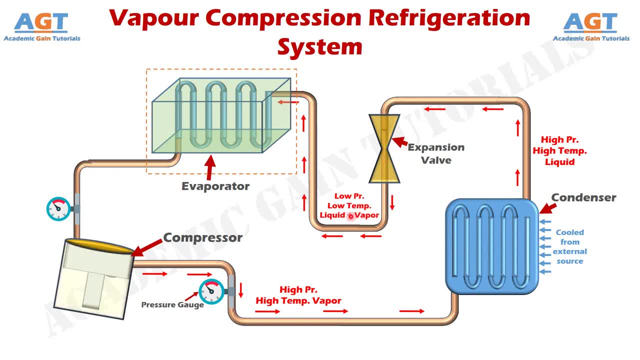 we do not get only liquid refrigerant, but here we actually obtain a mixture of low pressure, low temperature liquid and vapor refrigerant. Thus here we get a mixture of very cold, chilled, low temperature liquid and vapor refrigerant. Now we have a high pressure liquid refrigerant coming out of the expansion valve. Then